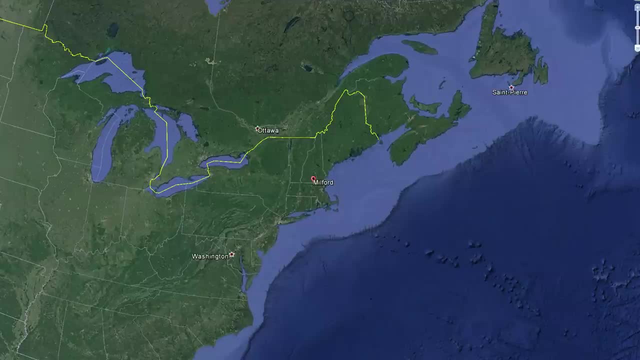 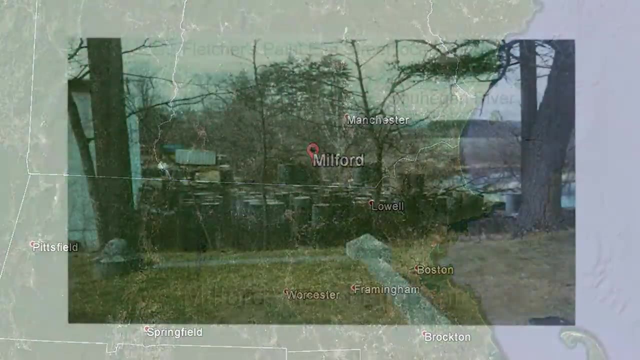 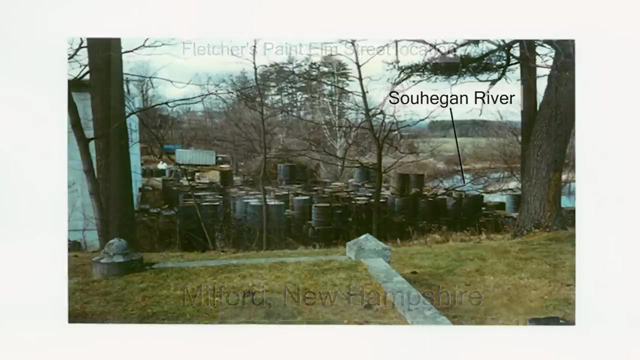 or the environment. In New England, where the American Industrial Revolution was born, legacy sites where chemicals were manufactured, used and dumped dot the landscape. What prompted everybody's attention towards the Fletcher Paints site was the Keys Municipal Well, Through routine environmental sampling by the state of New Hampshire and others. 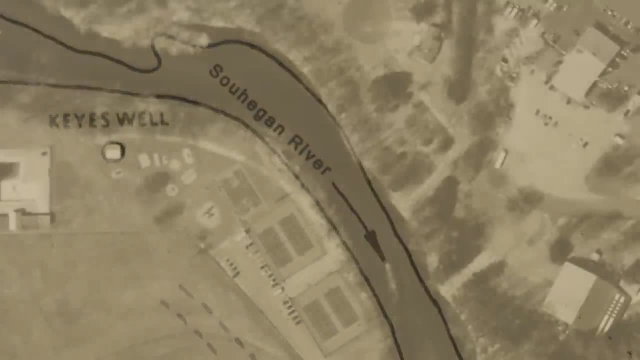 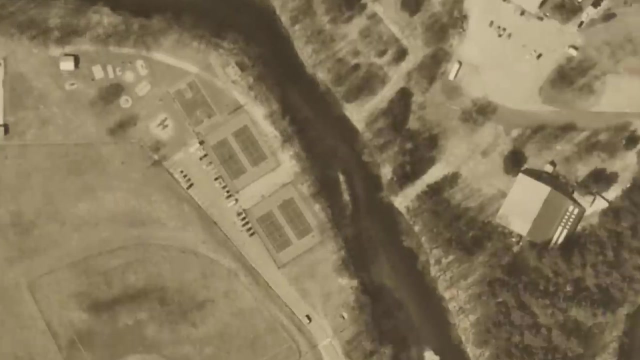 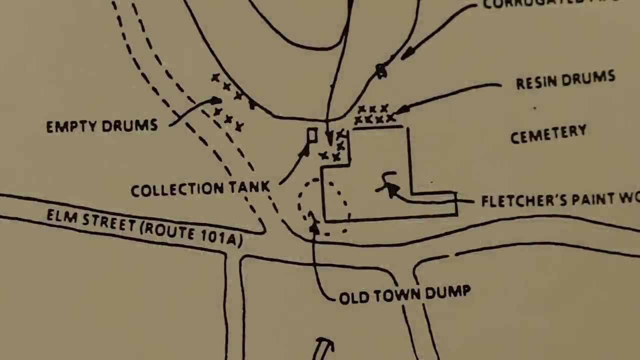 they found volatile organic contaminants in that municipal well, which caused a lot of problems because it provided drinking water for many residents in the town of Milford. They started to look for the contaminators and guess what Fletcher Paints? This site is unique. It had been an industrial site since the 1800s and there was a town. 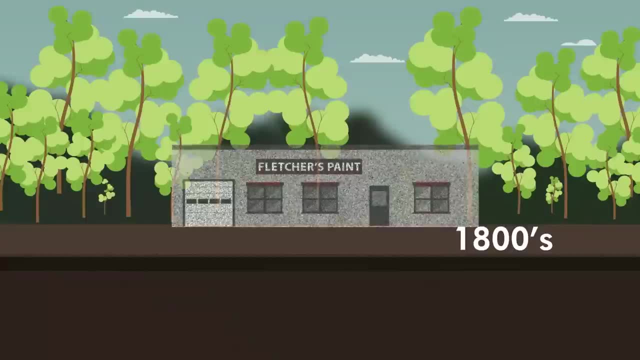 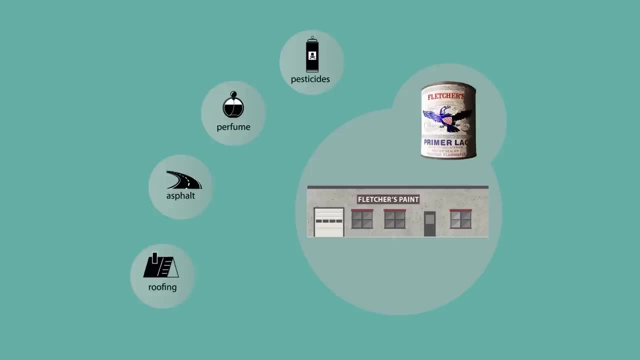 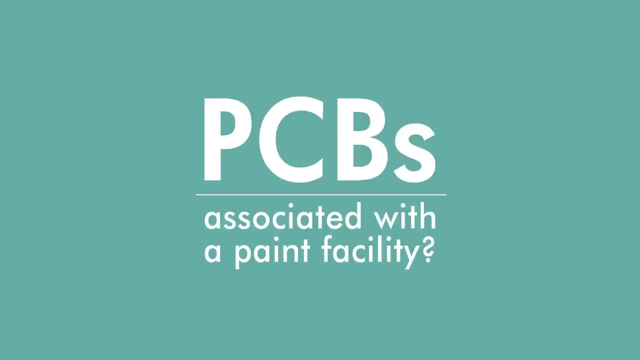 dump buried underneath it. The Fletcher Paint Company had some side chemical businesses. They made pesticides, they made perfumes and they made asphalt and roofing materials. EPA had to identify why there were so many PCBs associated with the paint facility, because it wasn't typical. It was discovered that 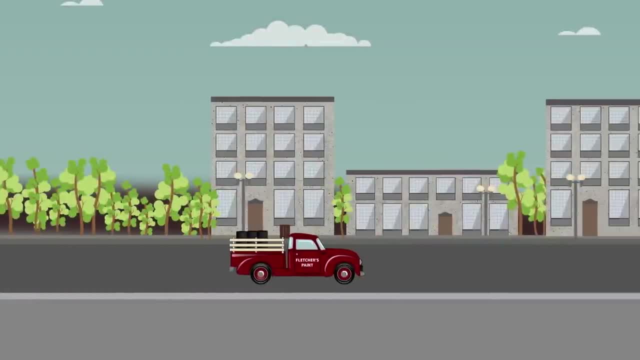 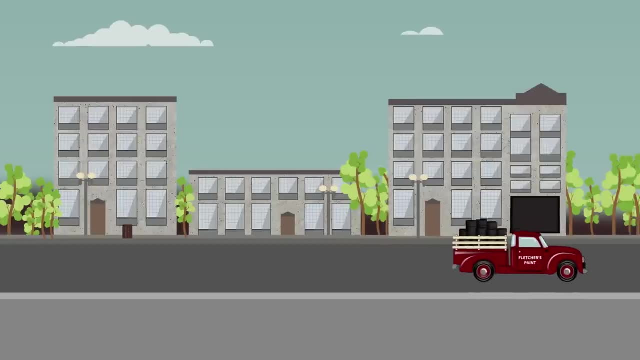 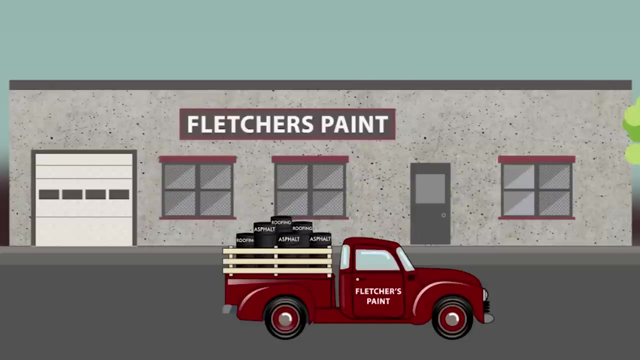 three companies were supplying a material called scrap pyranol, which is essentially a PCB material that comes out of capacitors or transformers. General Electric was Fletcher's largest supplier of this material. Fletcher's Paint was bringing the scrap pyranol in and shipping it out in products for asphalt and roofing companies. 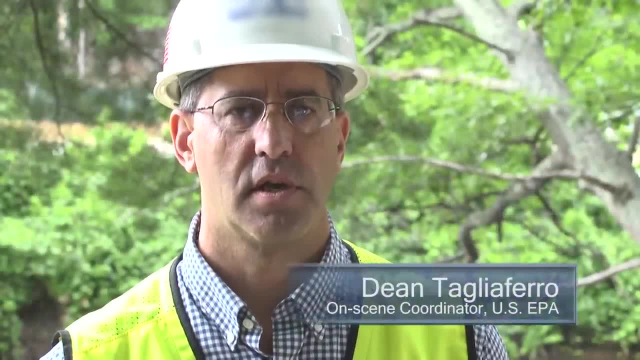 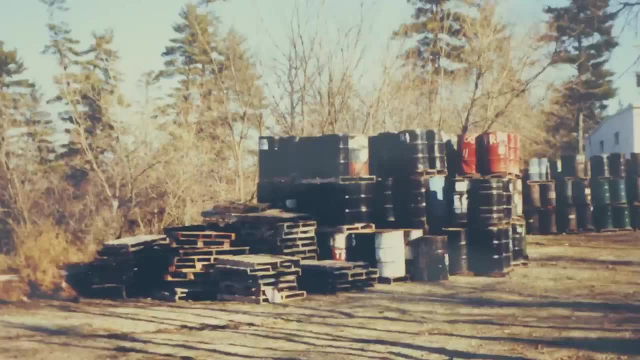 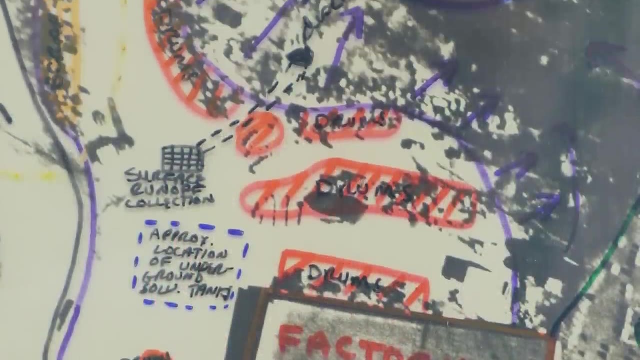 Unfortunately, they had about 800 drums of hazardous substances placed on the parking lot, which was a soil-based parking lot. The owners did not really know what the material was and the drums were slowly rotting and the materials were leaking out Very close to the river, so that was a threat to the 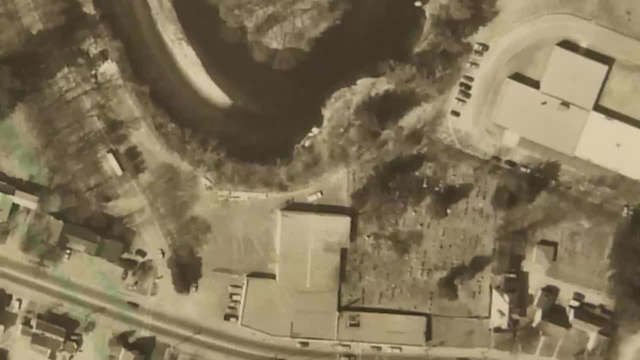 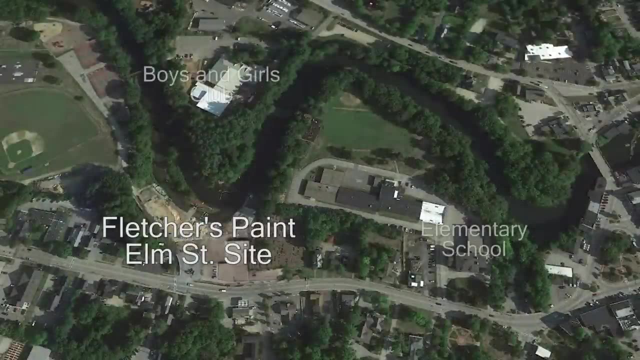 river a threat to the ground and the general area. This site is located near businesses, residences and an elementary school. The local Boys and Girls Club is just across the river. Once it was understood that Fletcher's Paint was a source of the contamination of the Keys, 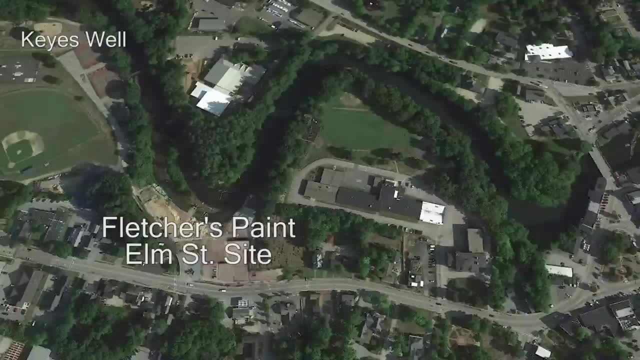 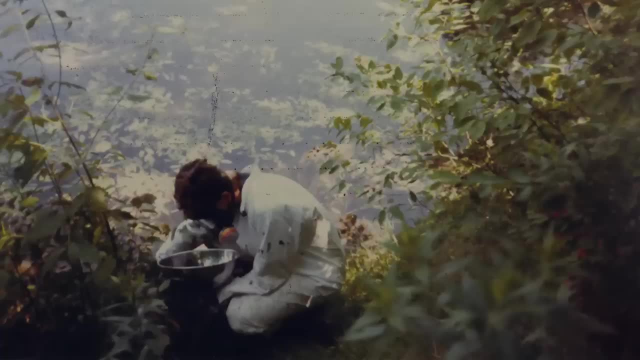 Municipal Well. EPA began working with the Fletcher Paint Company to find a solution. The Fletcher Paint Company began work to remove the leaking drums and conducted preliminary soil sampling. EPA did this work in 1988 via removal actions. Removal actions are typically short-term actions, about six months to a year in duration to 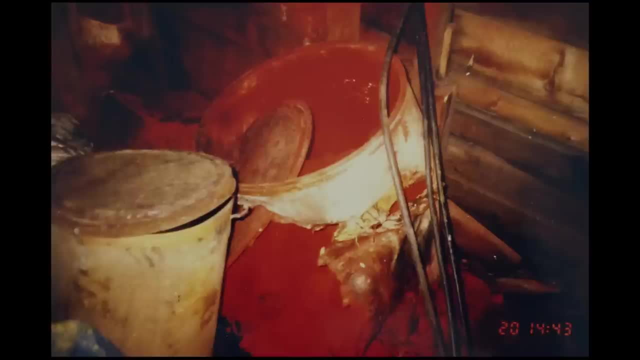 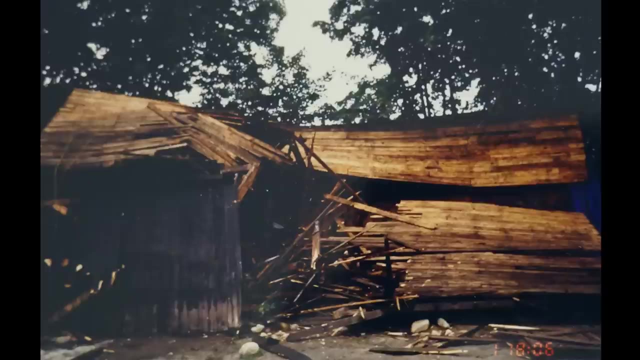 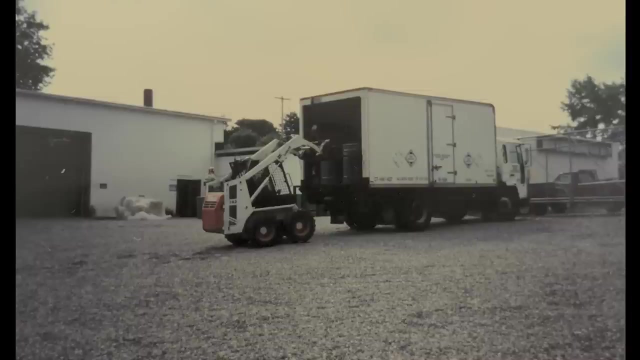 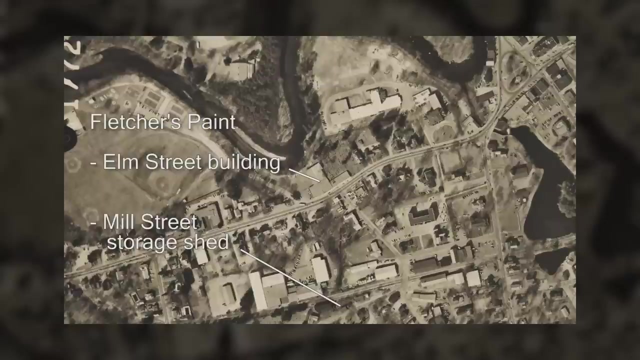 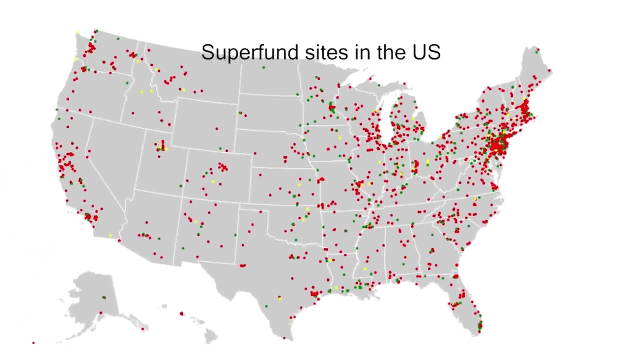 mitigate a more immediate threat. Removal activity in 1991,, 1993,, 1995, and 2000 also allowed EPA to address risks and manage building demolitions, fence installations and contaminated soil removal from residences near the site. Fletcher's Paint was listed on the National Priorities List, or NPL, in 1989.. The NPL 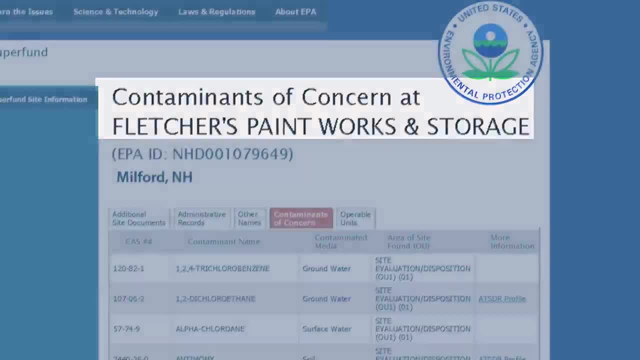 is another name for the Superfund program. Only the worst sites of pollution in America are ranked on the NPL and funds are available through Congress to clean them up. The NPL is the only place in the US that has a Superfund program, and only the worst. 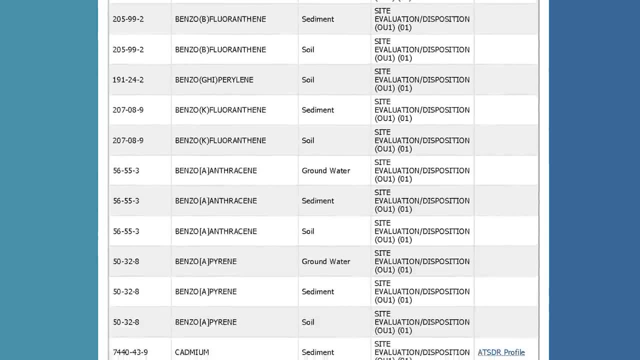 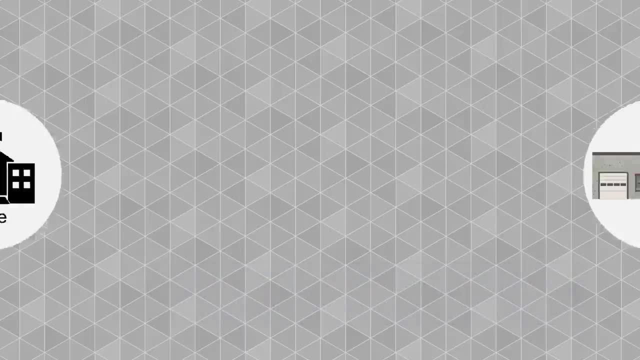 sites of pollution in America are ranked on the NPL and funds are available through Congress to clean them up. There's a number of entities that must come together in agreement to list a site for NPL. In a lot of cases a state discovers the site and assesses the magnitude of the problem. 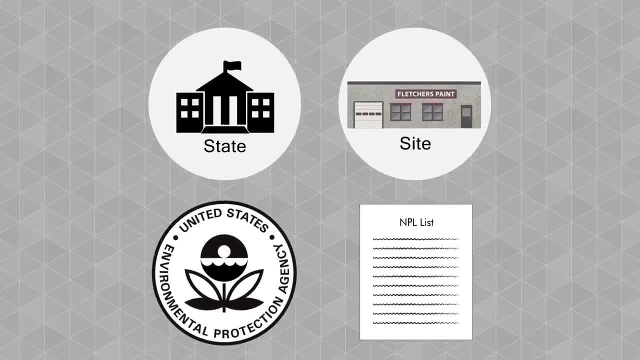 and, if deemed necessary, the state will refer the site to EPA and request the site be ranked for the National Priorities List. In order for a site to be listed, it must meet certain hazardous ranking criteria. There are many factors involved in this decision, including the types and levels of contamination. 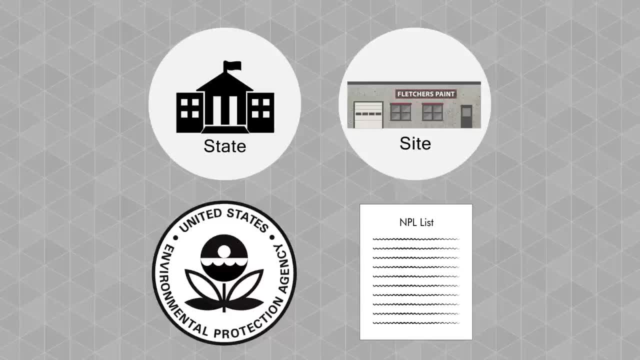 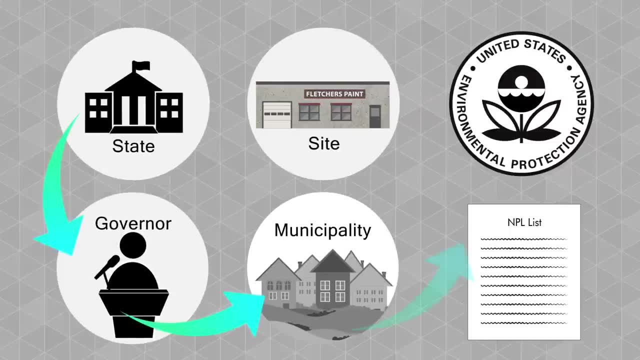 and their potential impacts. Ideally, the proposed NPL listing is supported by the governor of the state, the municipality the site is located in and community members there. Once a site is listed, the typical Superfund process will involve a lot of field work to 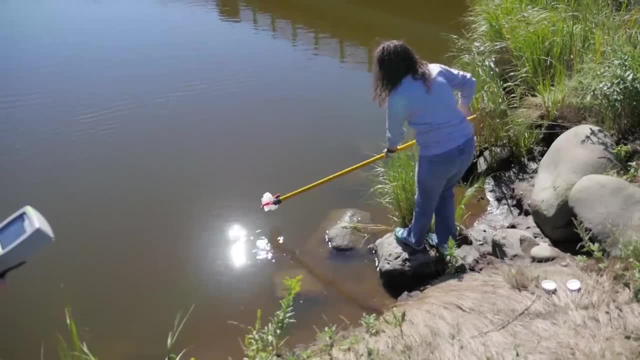 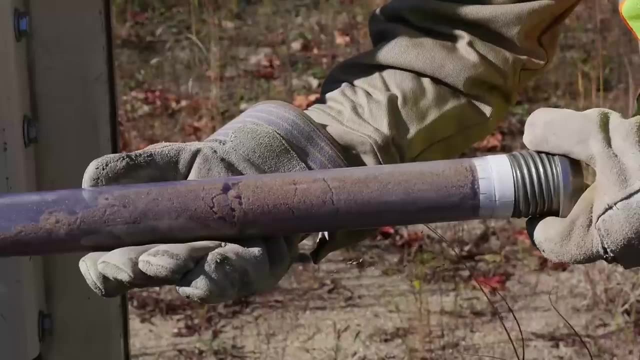 sample for the contaminants that may have been disposed of there- surface water and sediment sampling, soil sampling, ear sampling. That information is used to compile a document we call a remedial investigation, which summarizes the documents in the Superfund document. In the demonstration, the NPL list consists of only the most significant section of the last two years. The NPL will be listed in the Council for theanas in the Inclusion of the Statements, the National Priorities List, then theźniej list and the Kommunal Registration List. The NPL is listed in the National Priorities List and is listed in the National Priorities List. 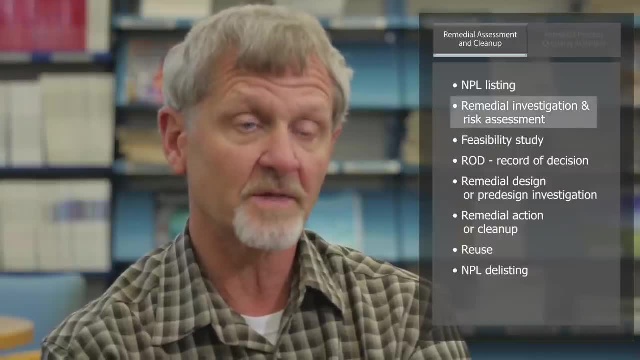 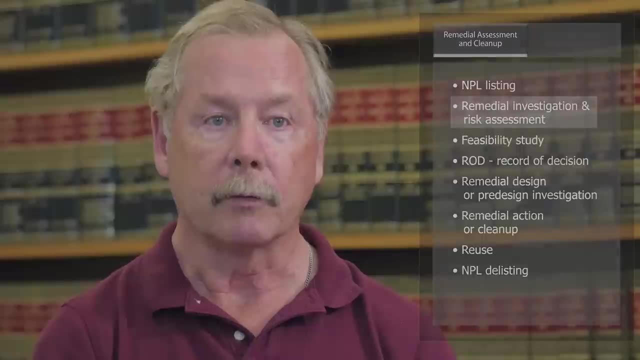 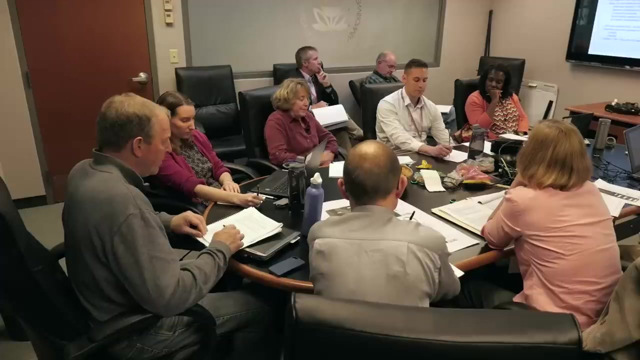 summarizes the contamination. As part of that remedial investigation we do a risk assessment. In the original scoping you try to figure out what receptors they're called, what people or animals will be exposed to the chemicals. We were concerned about cancer and non-cancer effects. 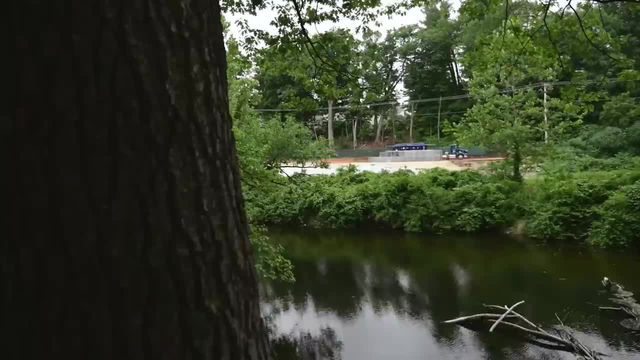 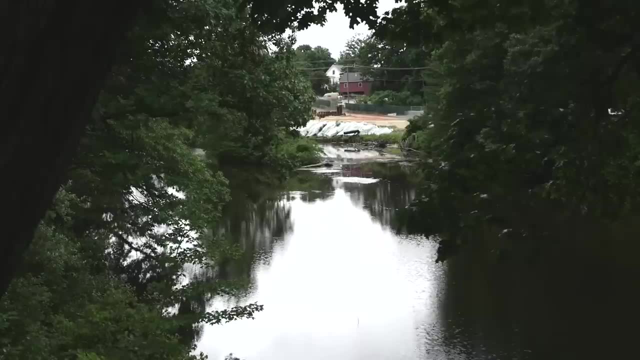 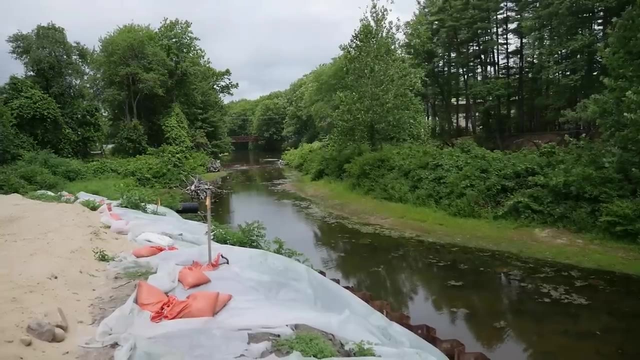 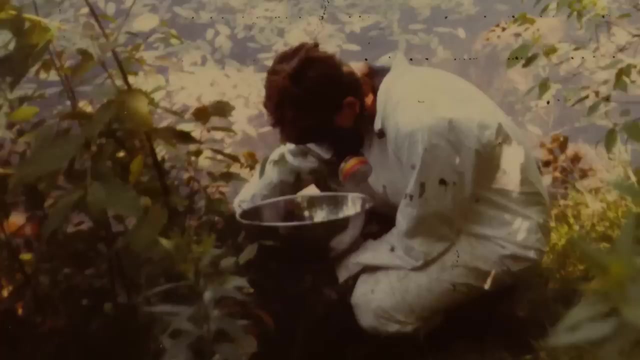 of the PCBs and some solvents as well, whether there were long-term chronic effects of these chemicals in trespassers, child residents, adult residents, construction workers. The ecological receptors were primarily fish in the river, so we looked at the effects on the animals themselves. 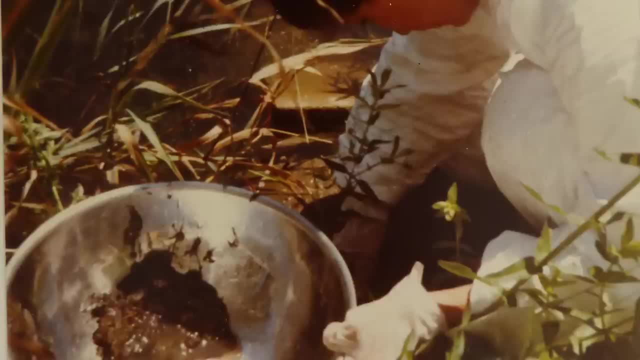 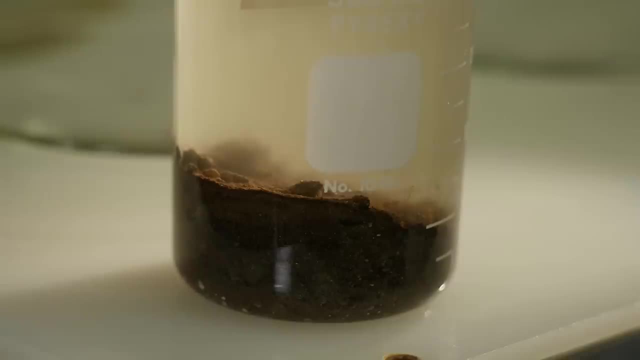 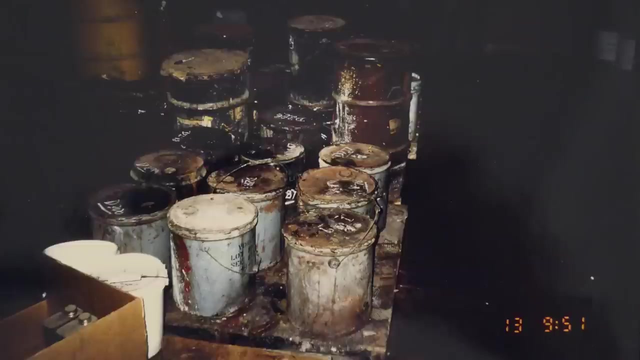 in the river and on wildlife or humans. The fish was a very important part of the research. The fish was a very important part of the research. The fish was a very important part of the research. So when they went out of business in 1991, they left behind a large building full of hundreds of drums and miscellaneous materials. 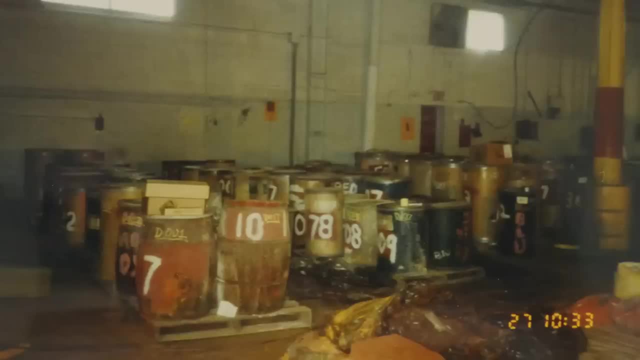 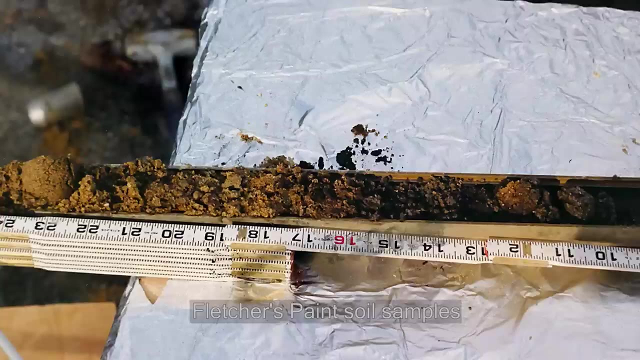 Because it was both a paint manufacturer. you could have an area of lead or antimony or chromium in one area of the site. You might have pesticides in another from that business. We never knew what the sample would show us because we never knew what may have been disposed of in a different area. 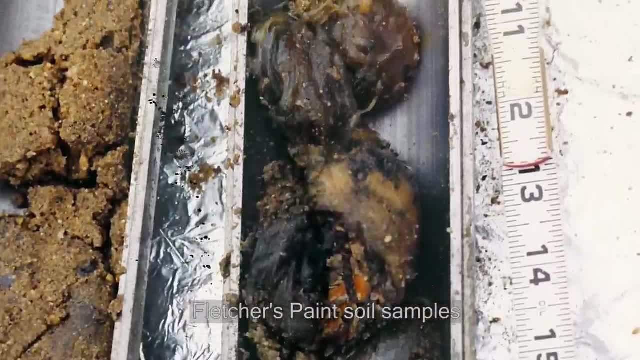 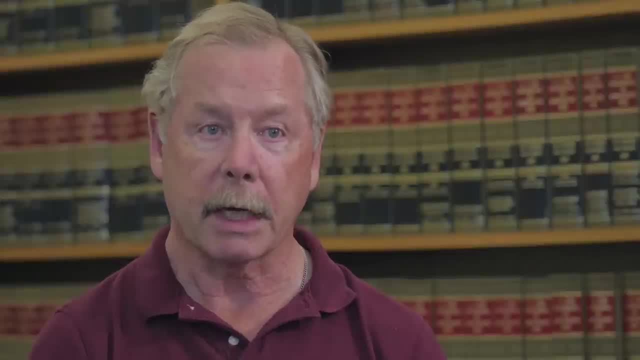 Remedial investigation is a very important part of the research. The investigation obtains the data, The risk assessor uses the data to calculate the risks, Then the engineers get involved in how much soil to take out. what is the method to remediate. 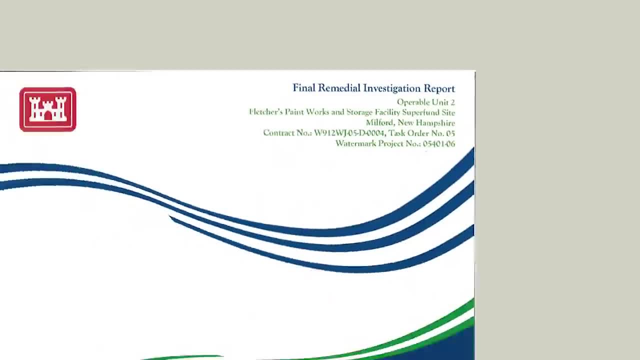 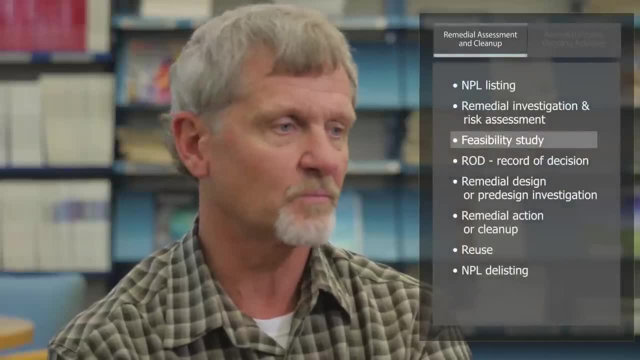 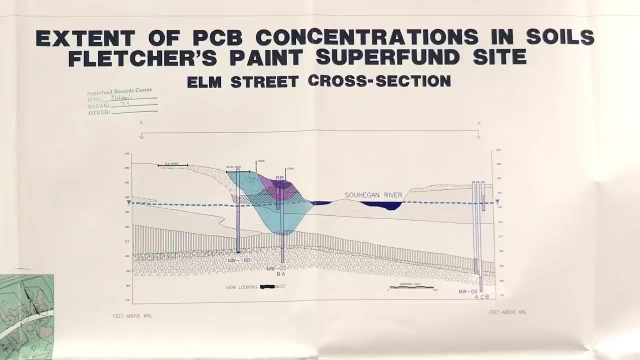 The remedial investigation serves as the basis for the feasibility study. The feasibility study will evaluate the various options that are potentially viable for cleaning up the site, whether it's soil or groundwater or sediment. That feasibility study then provides us the basis. It provides us the basis to propose a cleanup strategy. 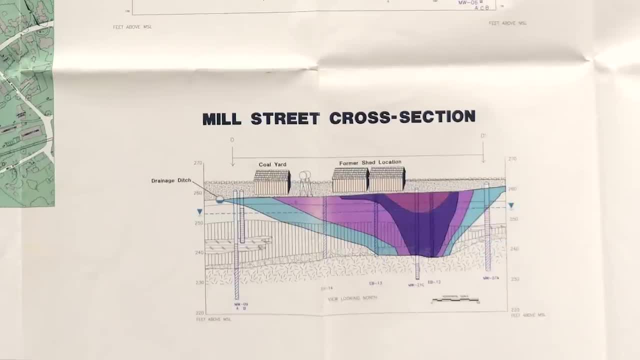 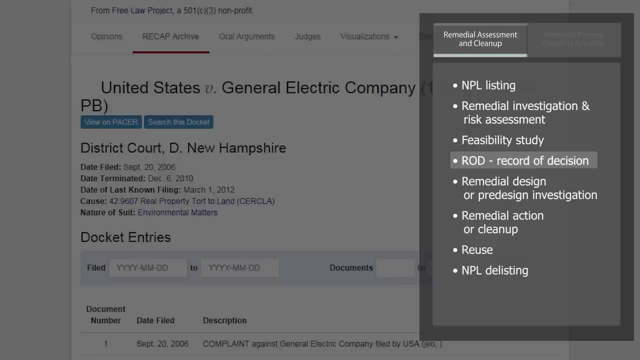 We have public comment on typically 30 days And then we write our cleanup decision or a record of decision that documents how to clean up the site. As the cleanup process progresses, EPA is tasked with other functions that move in concert to the cleanup. 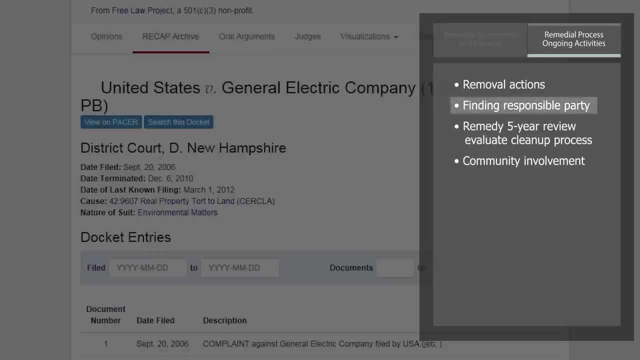 Part of EPA's job on Superfund sites is to ensure that polluters pay for the remediation of the site, which is done through EPA enforcement. EPA identifies the parties that are considered responsible- the parties that are considered responsible for the contamination under the law. 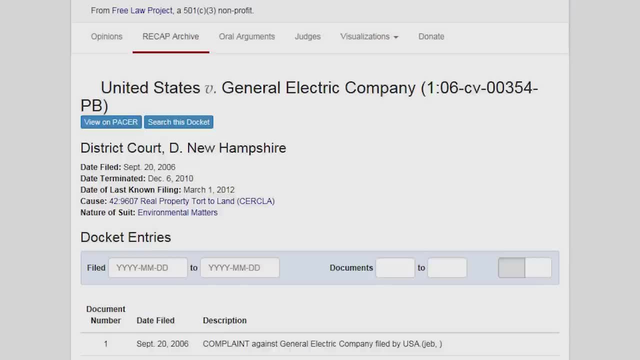 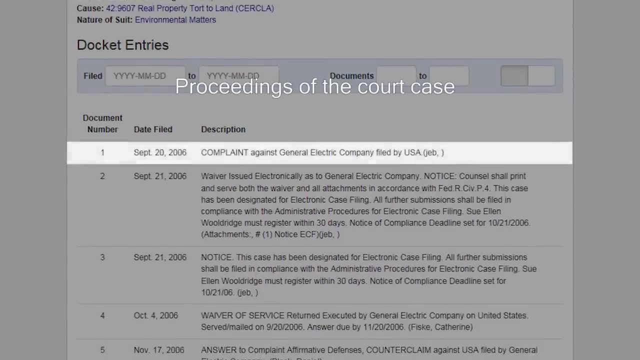 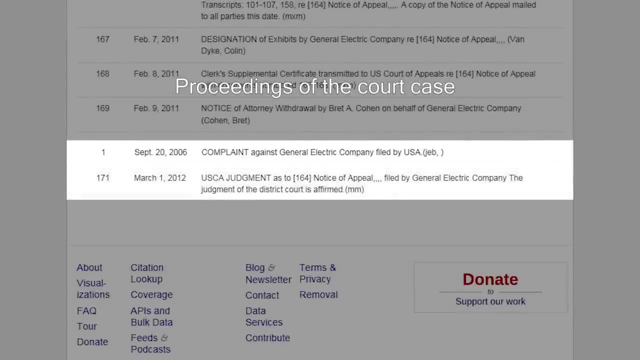 and asks those parties to perform the cleanup At the Fletcher's Paint Superfund site. EPA identified General Electric as the potentially responsible party, but GE contested. After the United States filed a lawsuit against GE, the company was found by the court to be a liable party. 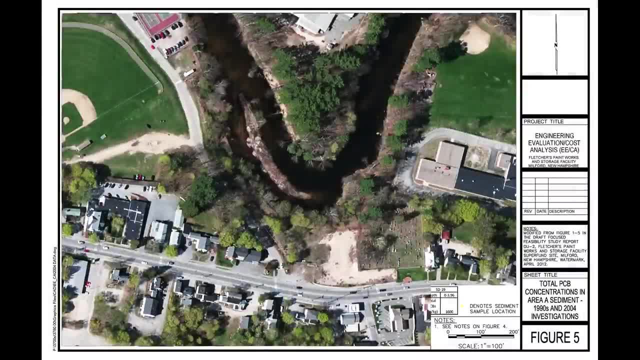 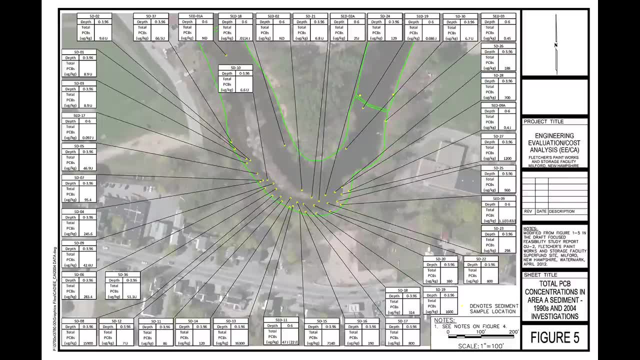 The second phase of the investigation is the pre-design investigations. That's pretty discreet. Instead of taking a few samples that shows high levels of contamination, you're taking 3,800 samples to look at very discreet depths of contamination. Where is it pooling up? 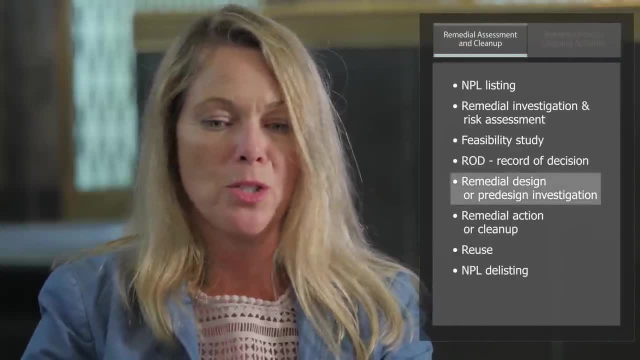 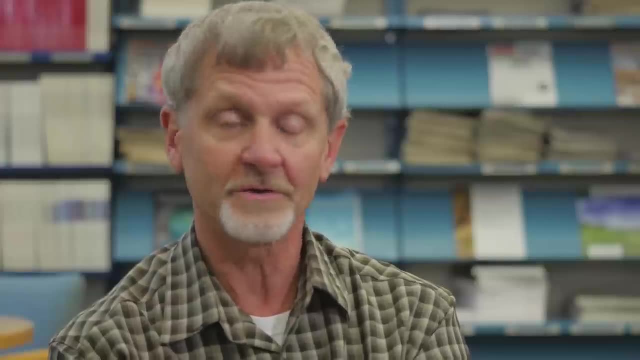 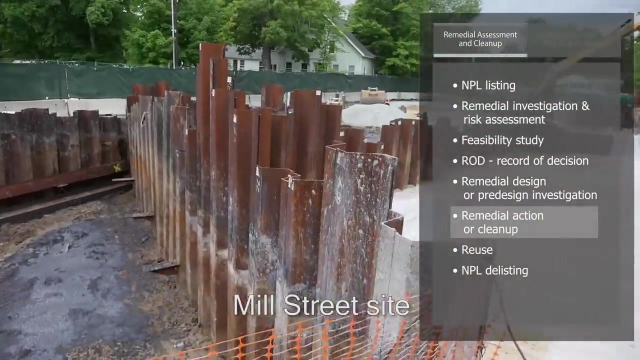 You're looking for how the data would respond to the cleanup. Basically, we try to do pre-design work to design the remedy that was selected and ultimately clean it up and perform the cleanup. The site is composed of two areas: the Mill Street site and the Elm Street site. 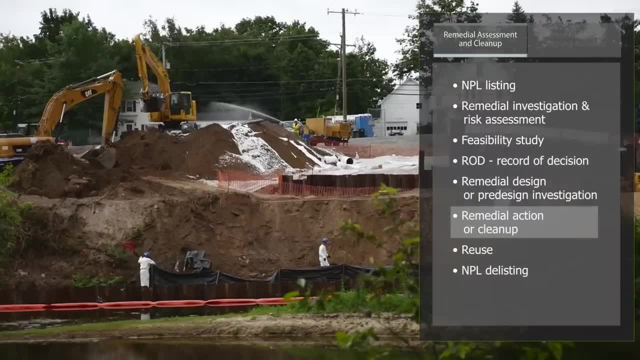 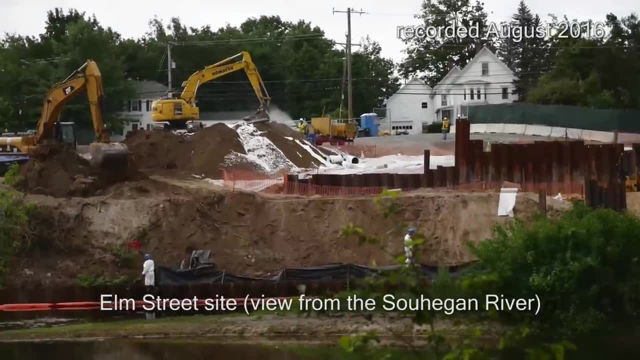 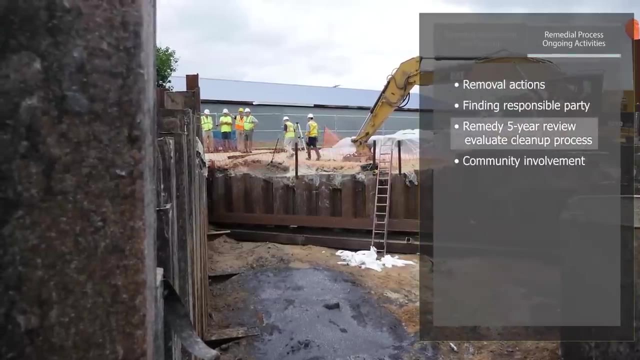 Both sites are in active remedial action currently for the removal of contaminated soils contaminated with PCBs being transported offsite. Some areas are going all the way to bedrock and other areas are shallower. The site is evaluated on an ongoing basis for remedy protectiveness. 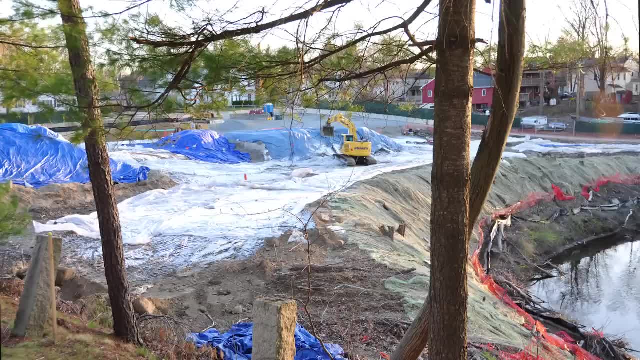 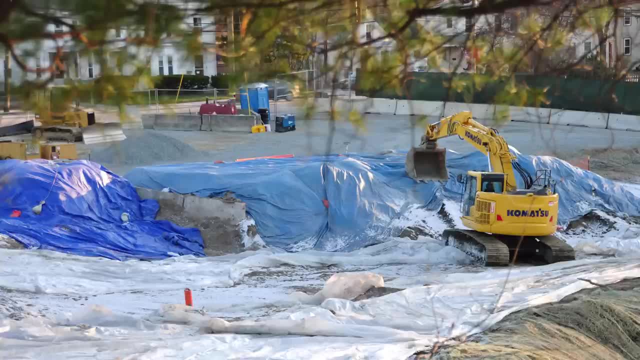 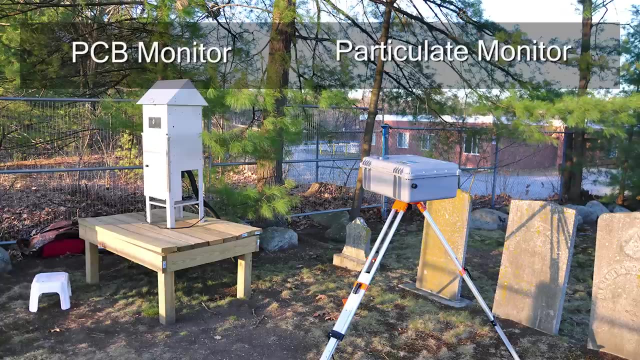 to make sure it still protects public health and the environment. During the early stages of the soil excavation we were detecting very high levels of PCBs in the air, much higher than the project action levels that were established. So we worked with the PRP, General Electric and their contractor. 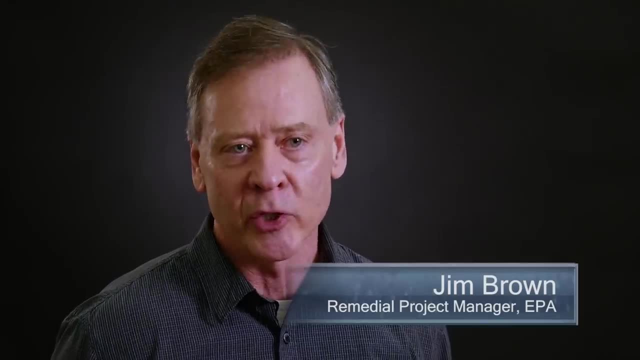 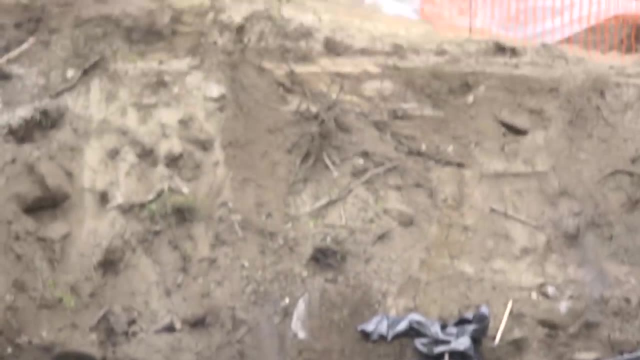 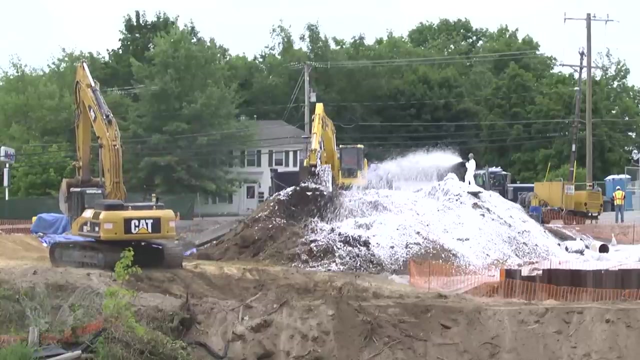 to figure out ways we could adjust the way we were managing the site. We finally wound up with developing a new plan. Part of that plan required additional engineering controls. Some of those controls included spraying vapor suppressing foam on the site. We also increased the amount of air monitoring that we were doing. 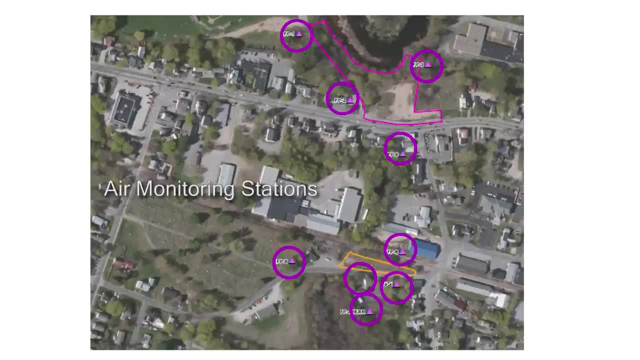 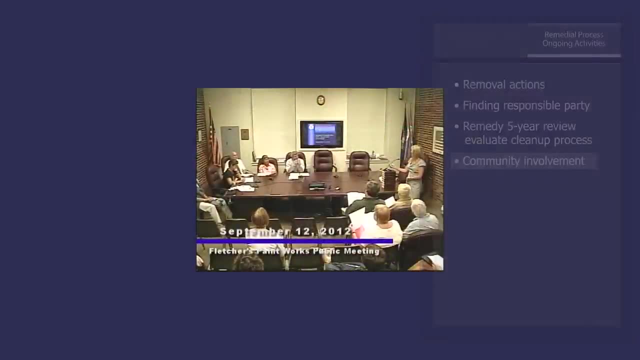 and the amount of air monitoring stations that were needed on the project. The community is encouraged to participate in the cleanup process and engaging the community is a focus of the cleanup team. We're going to start off tonight with a quick introduction. My name is Cheryl Sprague. I work with the Environmental Protection Agency. I am the remedial project manager for the Fletcher Paine Superfund site. With me tonight is my boss, Chief of the New Hampshire-Ride Island Superfund Section, Mike Jasinski. The work really couldn't be done without interacting with the community. 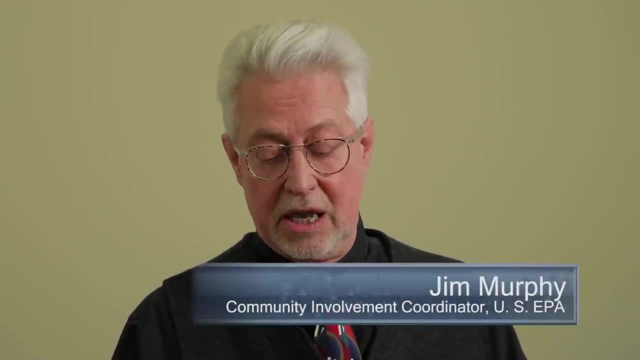 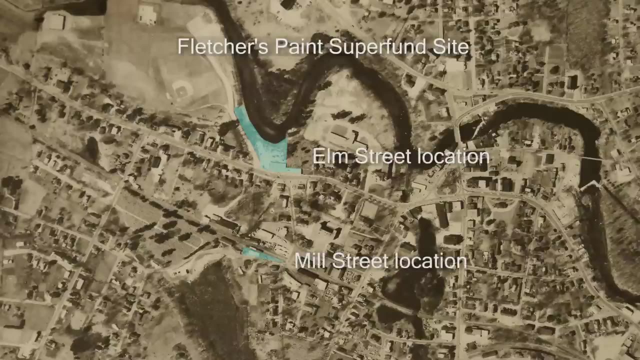 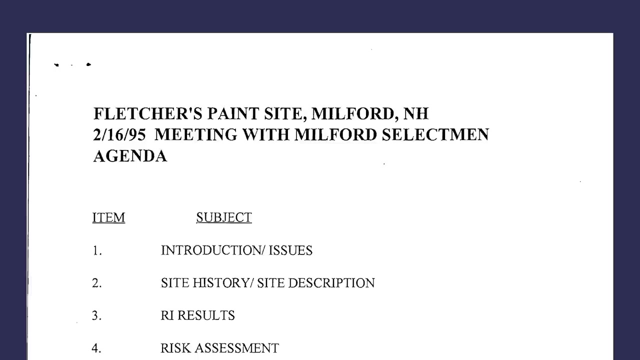 And on this particular site we were literally within six inches of people's front doors, front steps, and that's where the excavation was happening. I think the community involvement coordinator, besides dealing with the community, is also intensely dealing with the team.